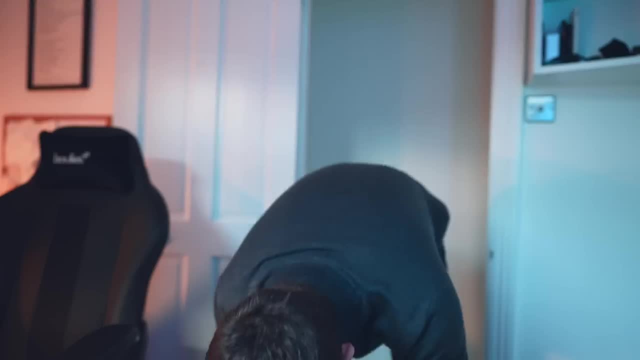 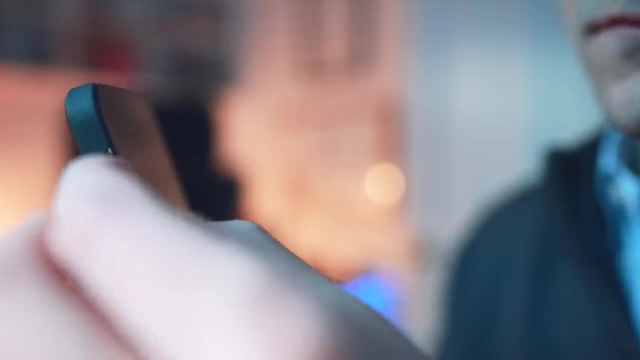 office or at home. I make sure I've been to the toilet, stretched my legs, got myself a drink and a healthier than I probably would at the cinema snack, And then also made sure that my phone is on, silent, not on. So I've been to the toilet, stretched my legs, got myself a drink and a. 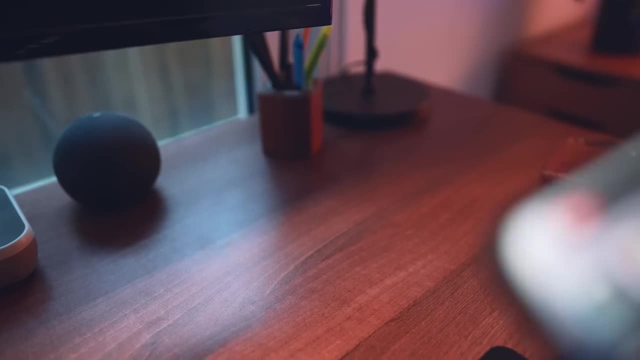 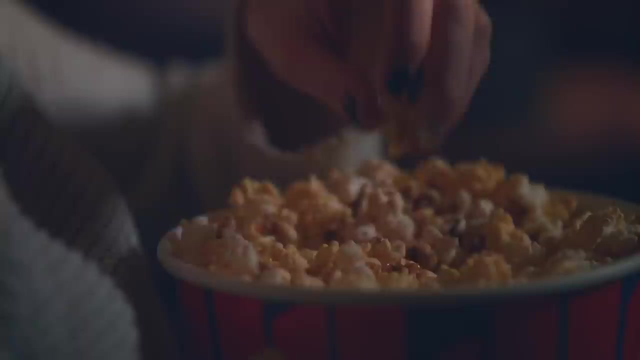 not going to disturb me. make sure that notifications or do not disturb is on allowing me to really immerse myself in the work that I'm about to do And just like when you're at the cinema, if you're like me and you find it hugely distracting and 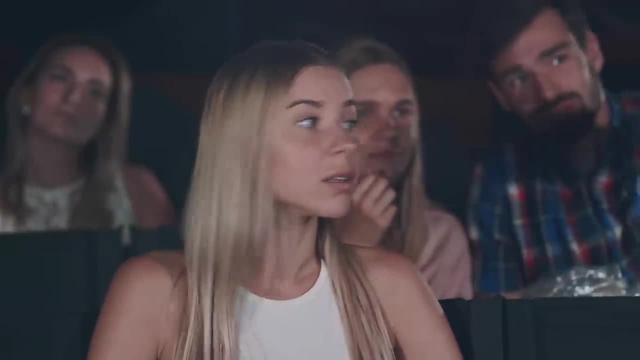 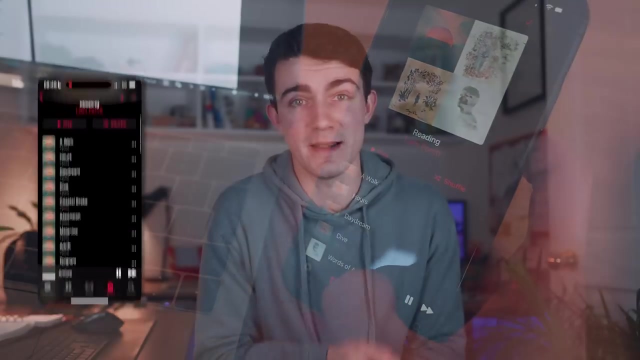 annoying when people are like rustling around in their popcorn and generally making noise around you, taking you out of that like state of flow of watching the film. I really strongly recommend that you use either a playlist or an app like Endel, today's sponsor. more on them later. 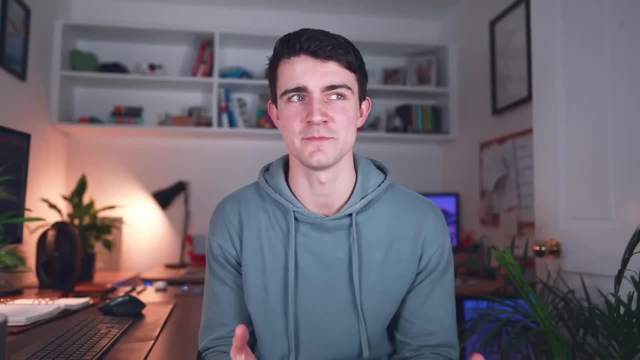 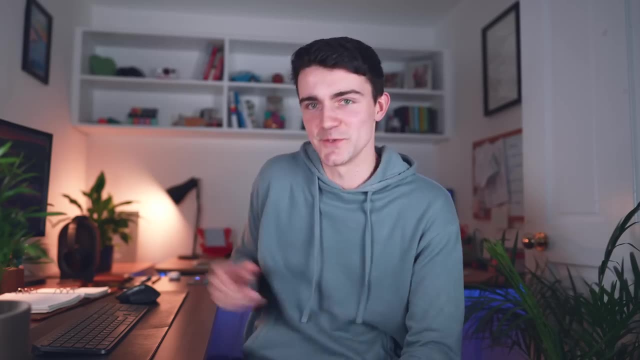 to really block out any distracting noise. This is so important for me that for when I'm in the office, I have my AirPods Pro with the noise cancelling function on. They're much more discreet than my bigger, Bose noise cancelling headphones that I wear when I'm at home. All of 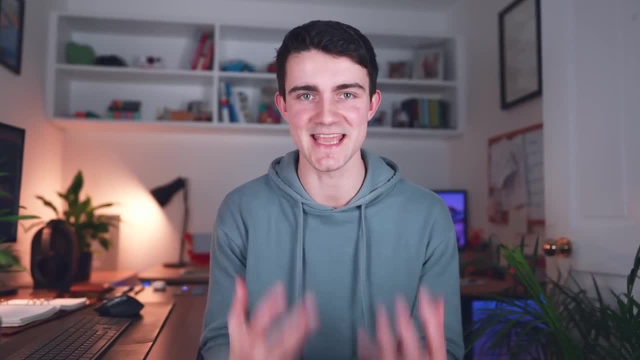 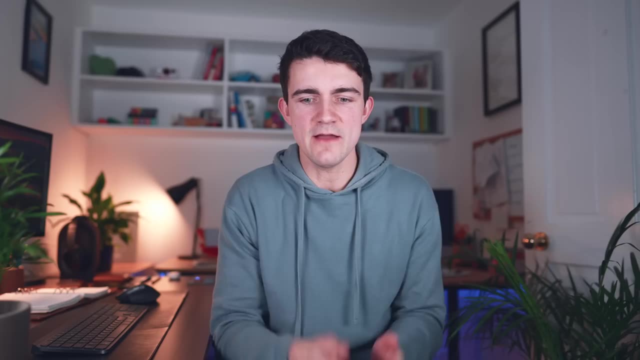 that then puts me in a state of mind where I am ready to get into a state of flow and immersion in the work that I'm going to do. The second habit is the batch task before you start. So batching is a very simple idea where, rather than switching between, I'm going to water this plant. 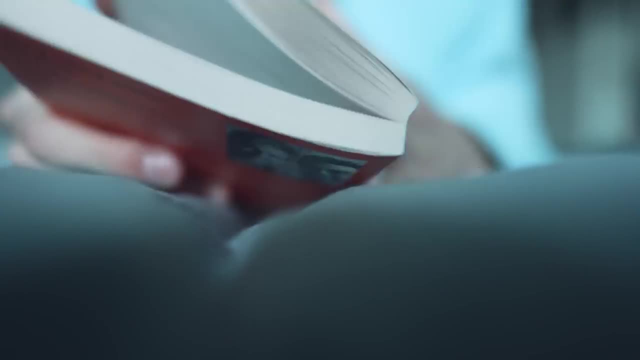 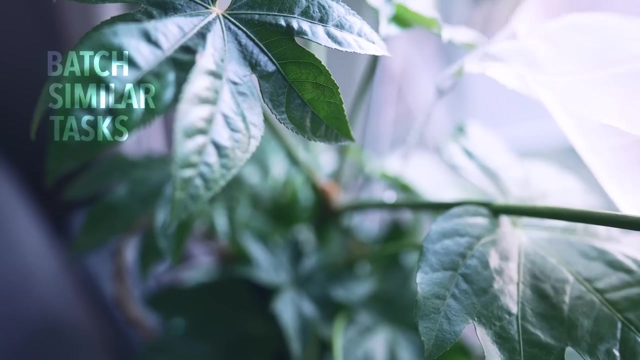 here, and then I'm going to do a bit of reading, and then I'm going to do some work, and then I'm going to clean the floor upstairs. You try to batch similar tasks. I'm going to do a bit of reading. so watering all of the plants at the same time, all at once, which just generally makes life way. 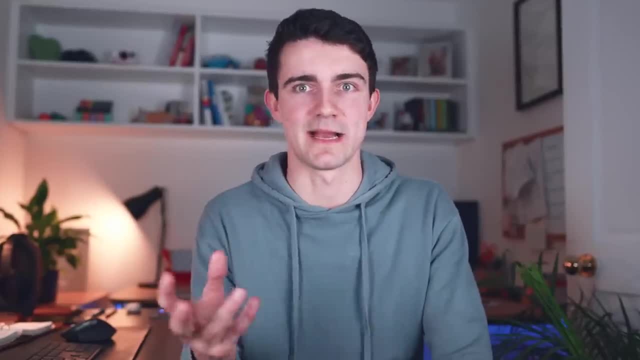 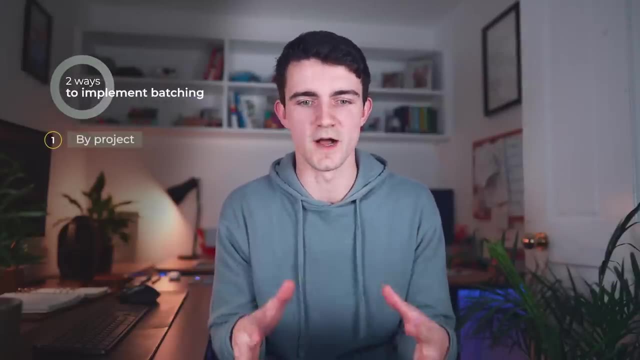 more efficient. I think the question here is really just like: how do I implement batching day to day? I think there are really two ways that I implement batching. The first is batching by project. What I mean by that is that when I'm at work and I'm working on, let's say something for 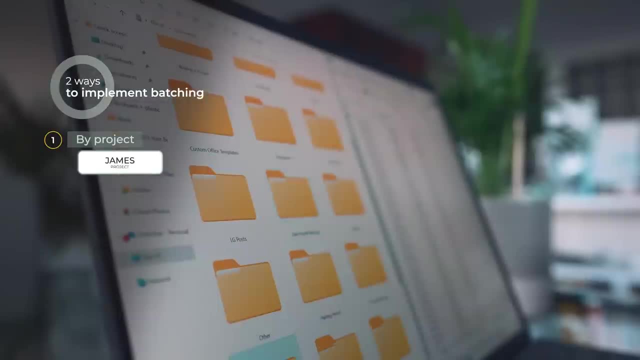 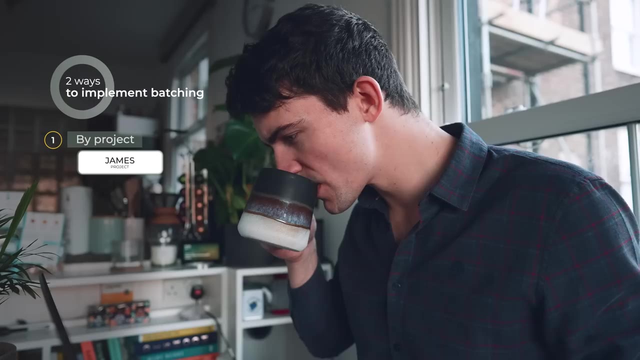 my client James. when I have all of the emails and documents open from James, it's way more efficient for me to do all of the work for James while I have everything there and open than it is to do something for James and then think, oh actually I really need to do that thing for. 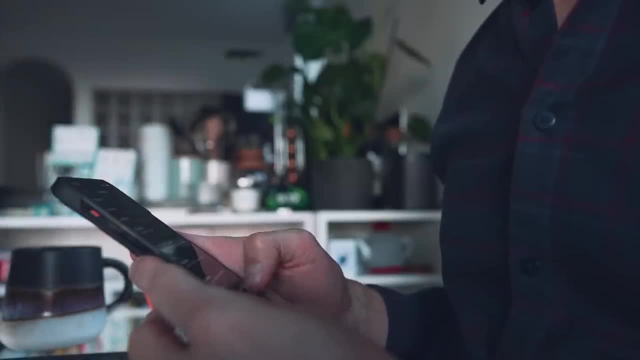 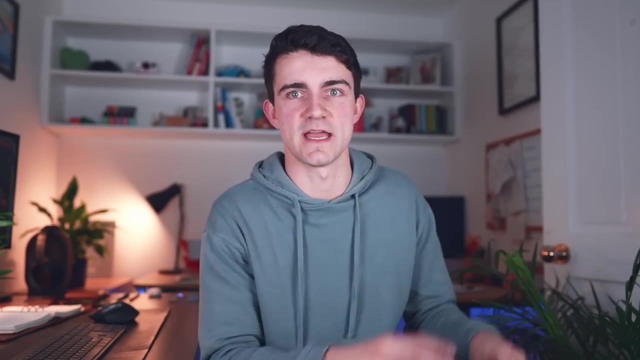 Sandra. So I'll just switch over and close everything and then need to open everything for Sandra and then open everything again for James later when I go back to James. Batching by project effectively means do everything for James and then everything for Sandra. It sounds pretty obvious, but I think actually being really conscious of when you are switching, 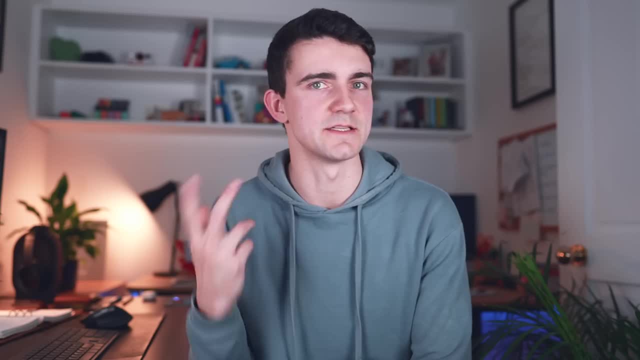 between projects way too frequently is a hugely healthy mindset to adopt. It allows you to be much more efficient in how you're working, both practically in terms of not having to open and close different things for different people, So I think that's a really good idea. 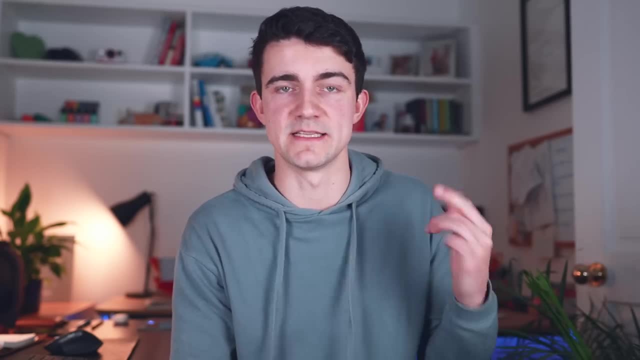 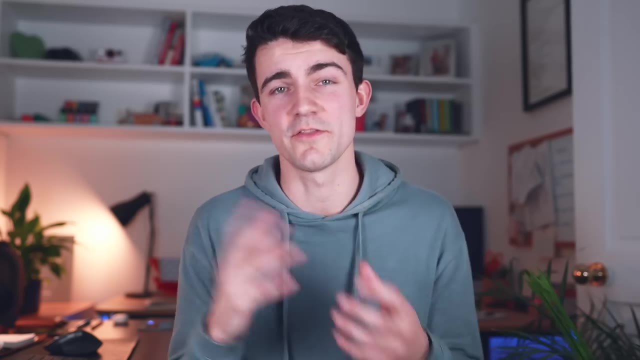 And also in terms of how your mind is operating. it is in the mindset of working for James, Do all of the work for James while your mind is focused and in that frame of mind, rather than switching between different projects. A top tip for me is when I'm at work and I'm working on, say three. 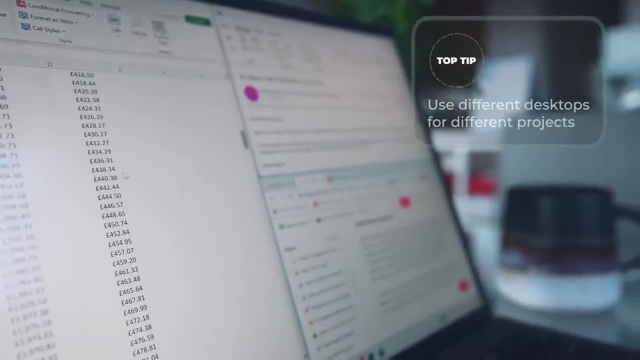 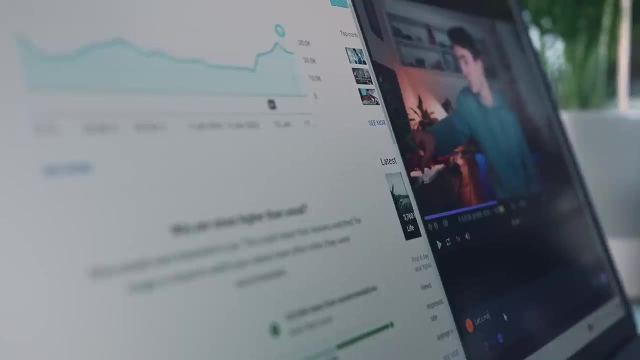 different projects at once. I actually have a different desktop for each of those different projects, So I actually have to move between desktops, which obviously allows me to keep all of the stuff relevant to a single project open in one desktop all at once And also creates 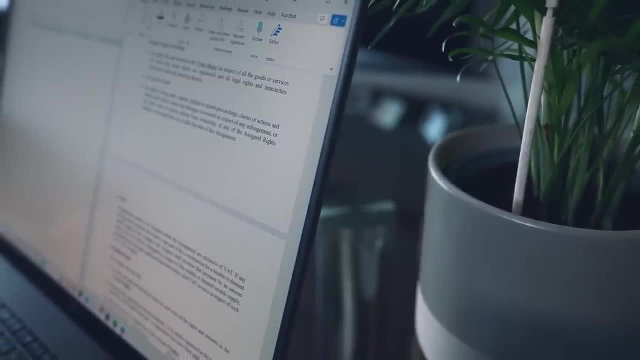 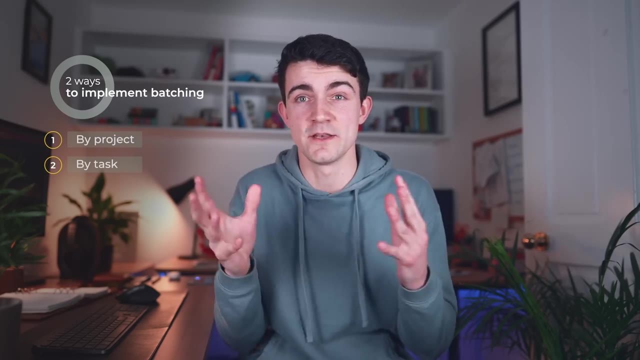 resistance for me in terms of how I'm working. So I think that's a really good idea. And the second kind of batching is just batching by task. So unless I get an insanely urgent email, I try not to reply to emails more than once every hour or two. So I'll let my emails build up and 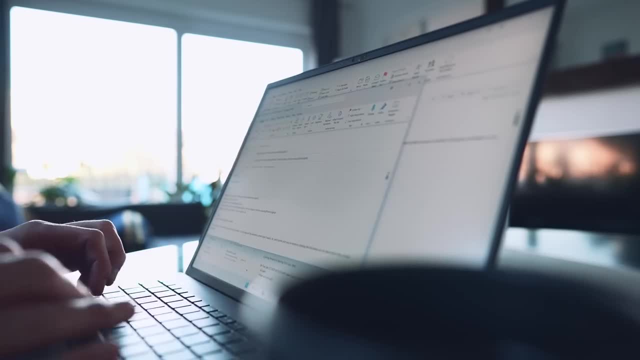 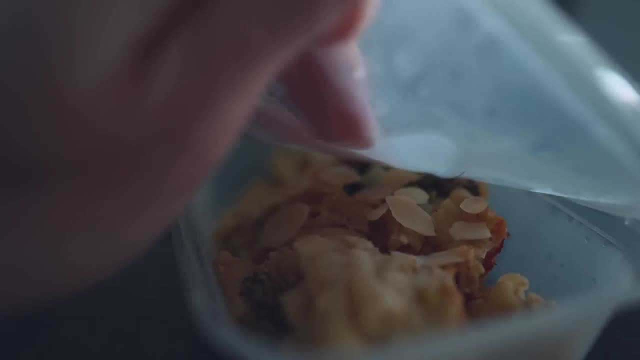 then do the task of writing and replying to emails all at once, And I also batch tasks outside of work. So, for example, when I'm cooking a meal, I'll make sure I cook two or three meals worth of that recipe, because it doesn't take massively more time to cook two or three times the amount. 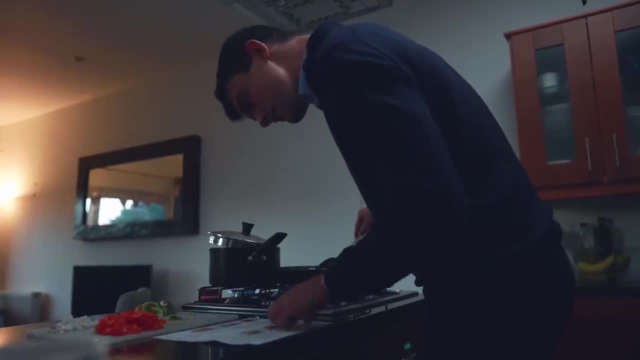 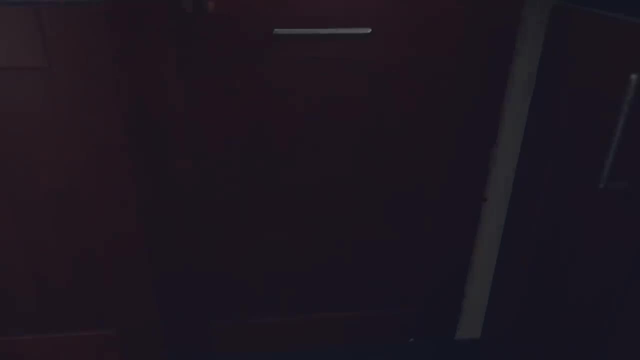 but obviously, if I cook a new meal every single night, that takes way longer, And I also batch chores. So if I'm cleaning, I'll clean the entire house for three hours rather than doing bits and bobs here and there. So yeah, for me, batching is really all about just having a consciousness of 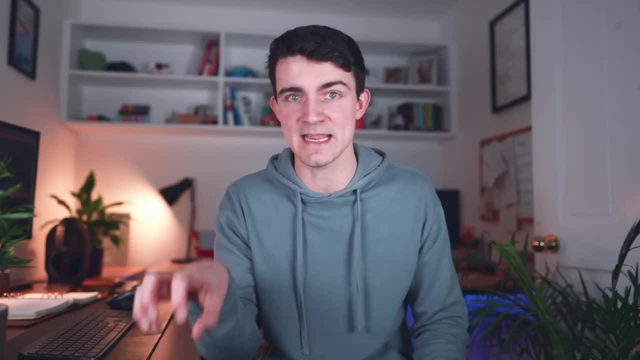 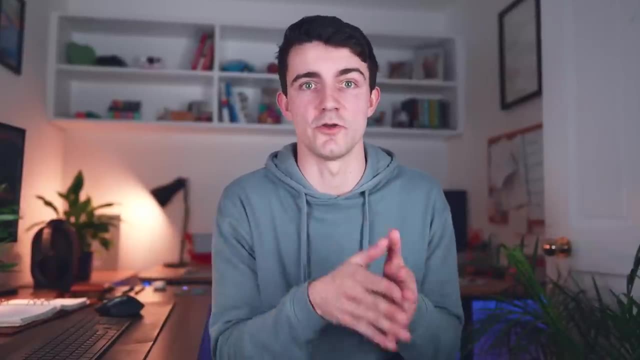 doing more of this type of task or this type of project right now, to avoid having to switch between things: losing focus and, overall, just spending more time than I should be on those tasks. So before we move on to the final two habits I really quickly want to tell you about 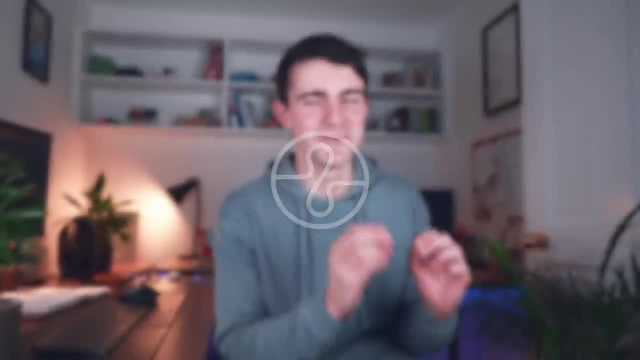 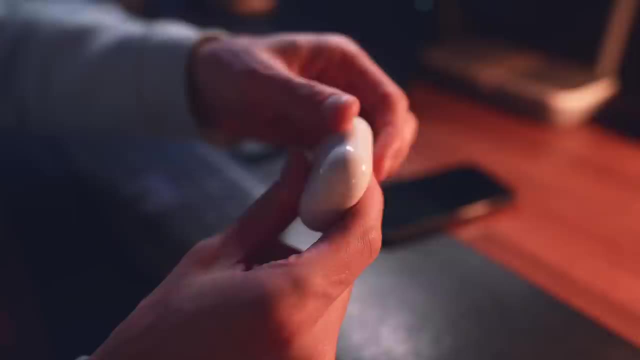 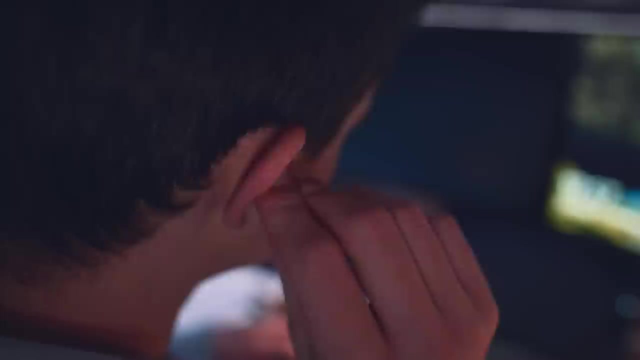 today's sponsor, Endor, Which has pretty quickly become probably my most used app. It creates personalized real-time soundscapes that help you focus, relax or sleep, So Endor is, without a doubt, the single best app I've ever had to get me in the zone whenever I'm finding it hard to concentrate on work. 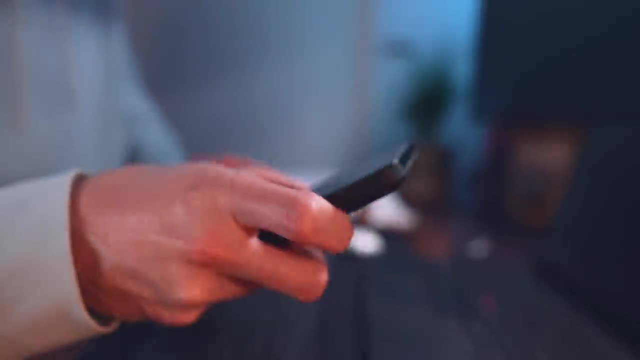 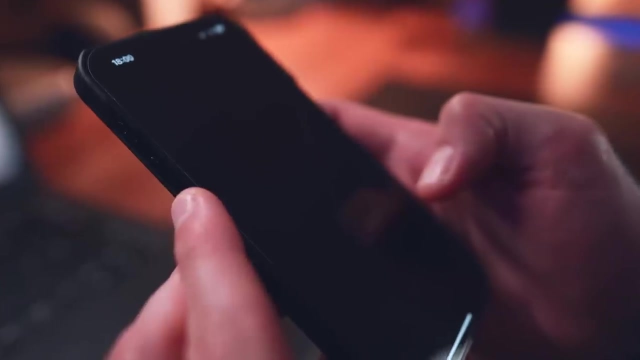 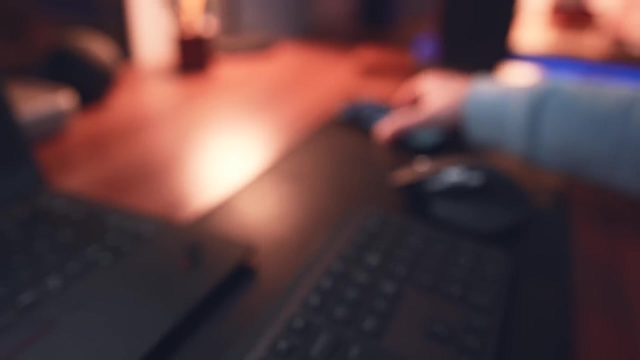 especially if there's background noise where I'm working, which I'm particularly bad at blocking out. Endor is informed by science, created with science and backed by science. It's an environment-based app that takes everything we know about sound to create real-time, personalized soundscapes that help with focus, as well as relaxation and sleep. 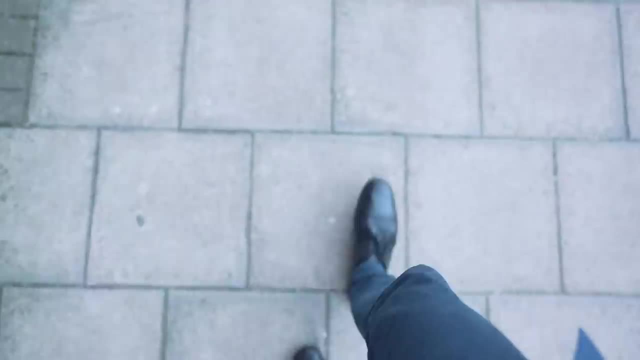 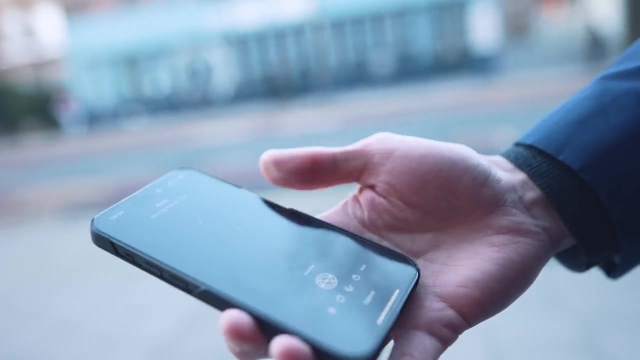 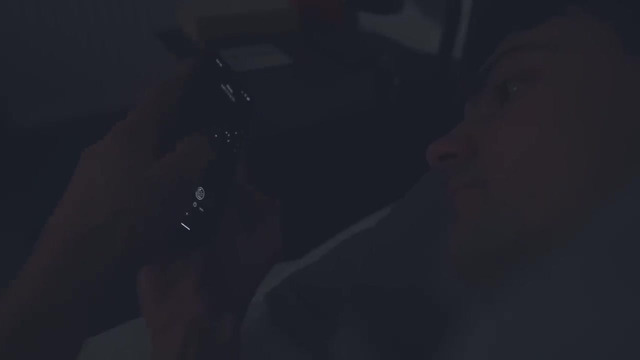 I genuinely find Endor complements my body's natural circadian rhythms, using its AI-powered technology to help me relax when I'm stressed. I always listen to Endor's relax mode on my way home from work when I've had a tough day, or to reliably get me in the mood to sleep even when I 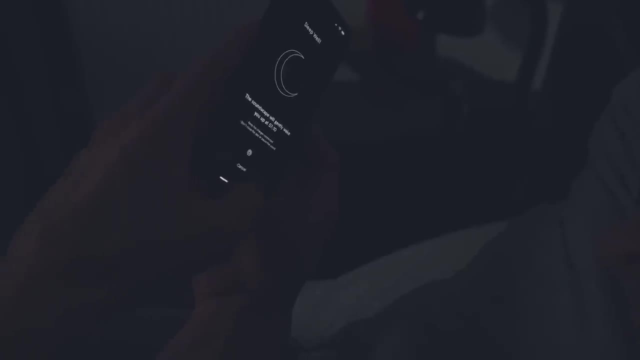 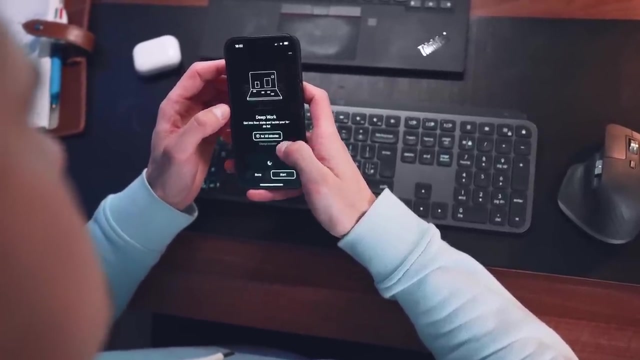 feel a bit restless. I absolutely love their gentle alarm that slowly wakes me up in the morning, rather than that we all know and hate, And I'm also a huge fan of Endor's scenario mode, which allows me to tell the app: okay, I'm going to do deep work now. I'm going to do it for 60. 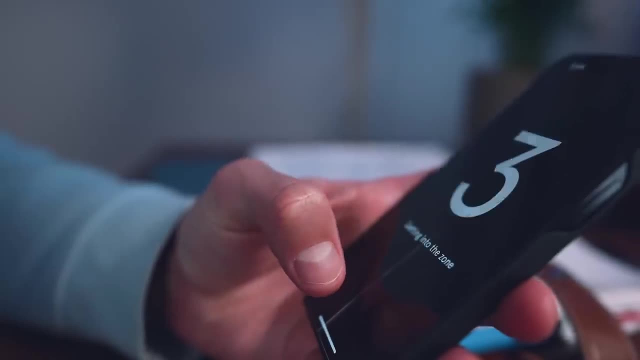 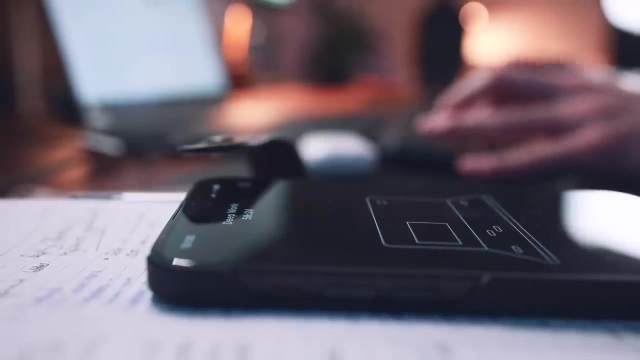 minutes and then I get a soundscape to help me get in the zone for that entire work session. So if you want to start using Endor's amazing soundscapes that keep me focused for hours, pretty much every single day, follow the link in the description and the first 100 people to download. 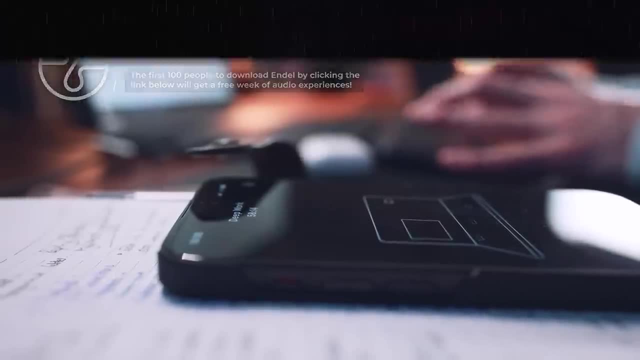 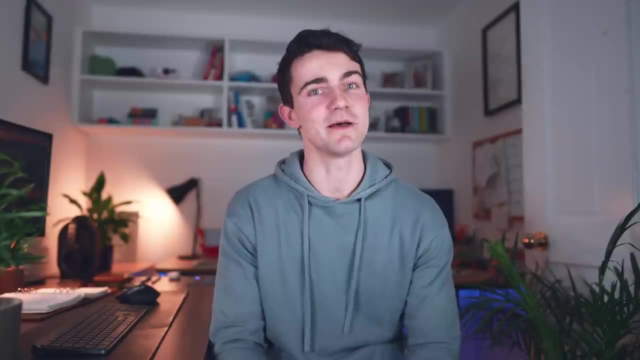 Endor will get a free sound. So if you want to start using Endor's amazing soundscapes that keep free week of audio experiences, Alrighty. third habit is to try to avoid work before doing the work, And this is inspired by Grace Beverly's book Working Hard, Hardly Working. So there 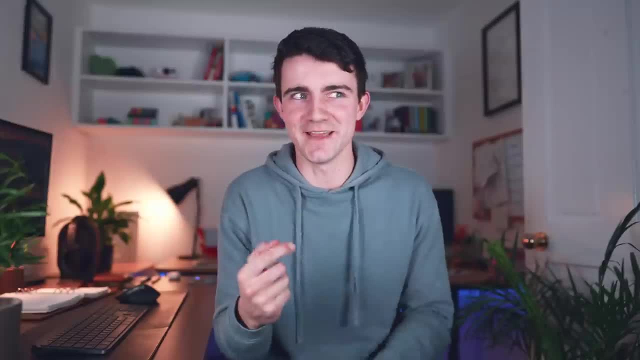 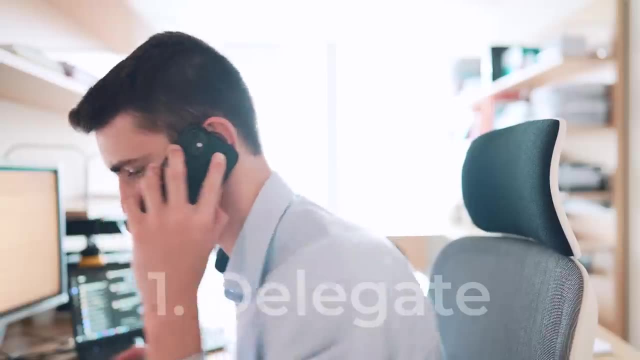 are two ways that I try- and I think anyone can try- to avoid doing work myself in order to have more time for other stuff. The first is to delegate. I think in a work context it's so easy to be given a task to instantly jump into doing it and five hours later you've finished. 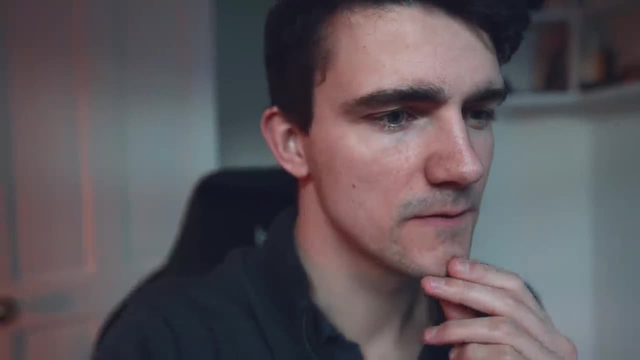 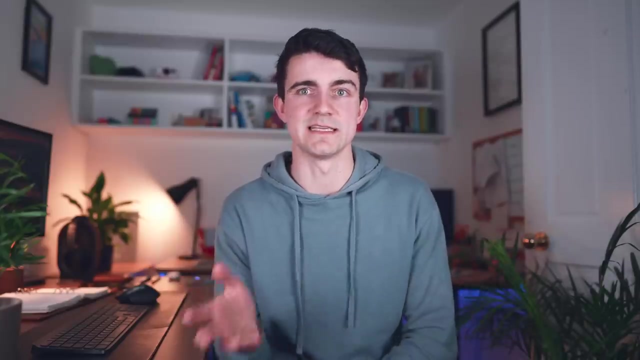 So for me, the habit is really just spend five minutes thinking before I jump into this task. are there other people who can more effectively do this than me? Are there people who could help people with more expertise in this area than me? I really do. 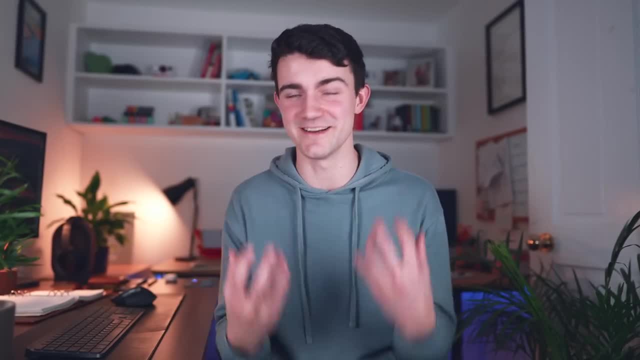 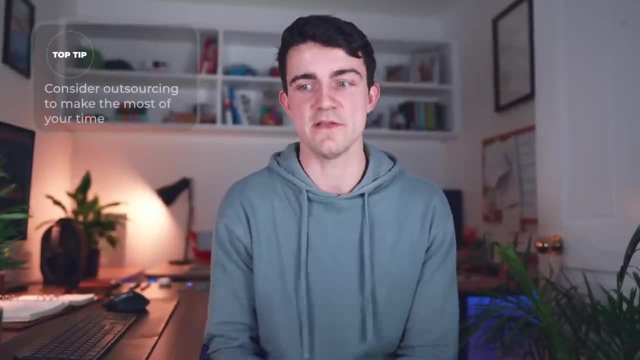 genuinely find it so tough to delegate because I'm quite protective of my work. I really want the work to be high quality, but I think getting into a habit of considering options to outsource is absolutely critical if you want to make the most of your time. And the second is to use tech.